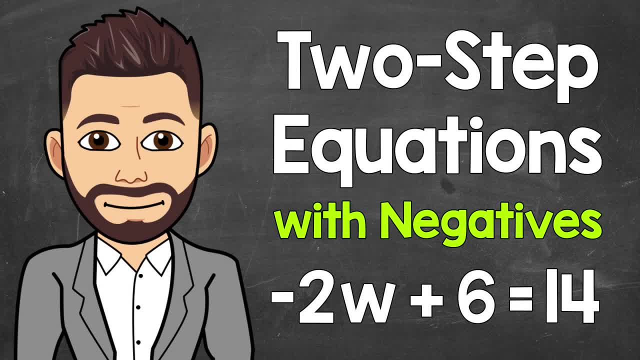 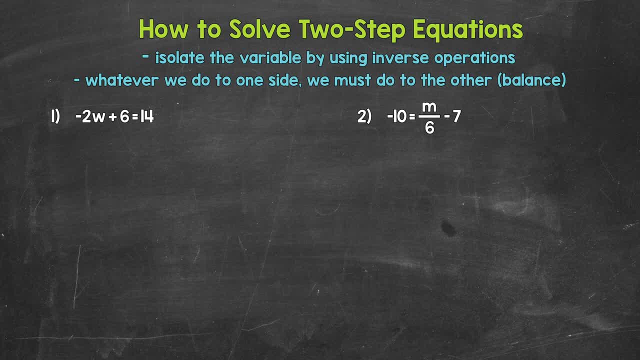 Welcome to Math with Mr J. In this video I'm going to cover how to solve two-step equations involving negatives. Now remember, when we solve equations, we want to isolate the variable, And we do that by using inverse operations. And whatever we do to one side of the equation, we must do to the other side of the equation. 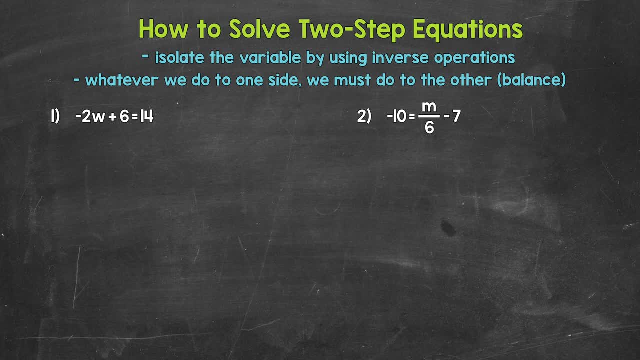 Now, when we have equations that involve negatives, we need to be careful and work through everything correctly as far as the negatives go. So let's go through and take a look at a couple of examples here and see what we need to keep in mind when working with negatives. 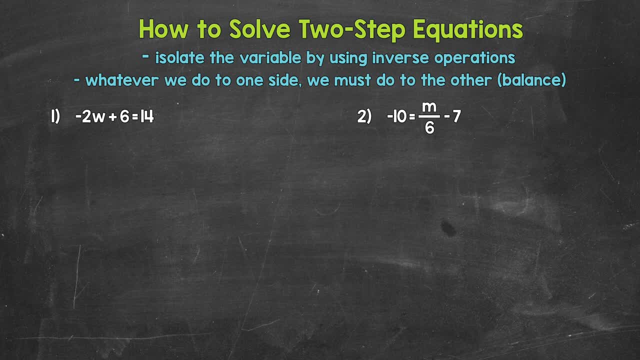 Let's jump into number one, where we have negative 2w plus 6 equals 14. So negative 2 times what plus 6 equals 14. We need to isolate that variable of w by using inverse operations And we will go in the reverse order of operations. 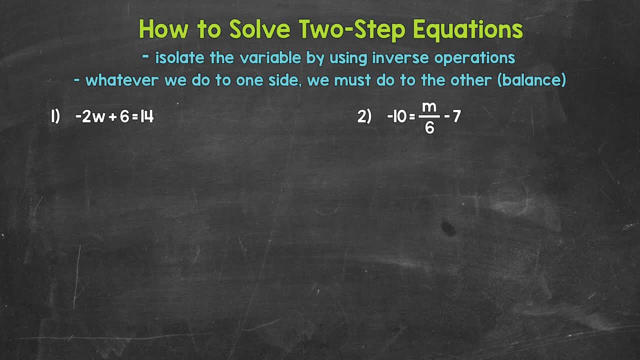 So we need to undo the addition first. What's the inverse operation of addition? Subtraction. So we need to subtract 6 from the left side of the equation. Whatever we do to one side of the equation, we must do to the other. 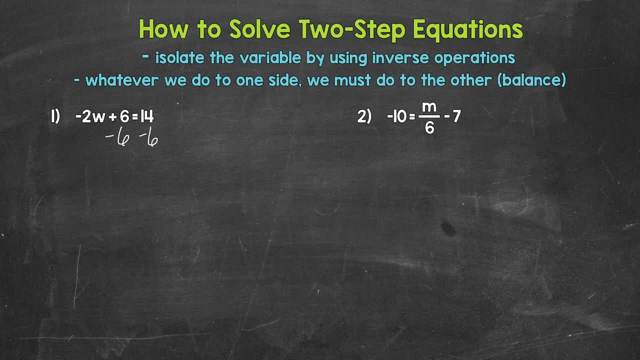 So subtract 6 from the right side as well. Now on the left side of the equation we are adding 6 and subtracting 6.. So these 6s cancel each other out. So we have negative 2w equals. 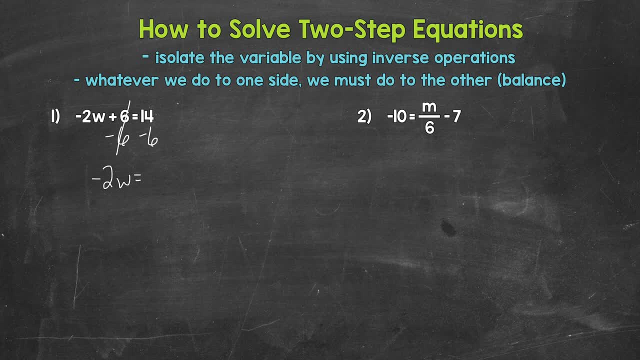 And then on the right side of the equation, 14 minus 6. That gives us 8. So we have negative. 2w equals 8 now. So we are multiplying w by negative 2. We need to undo that multiplication. 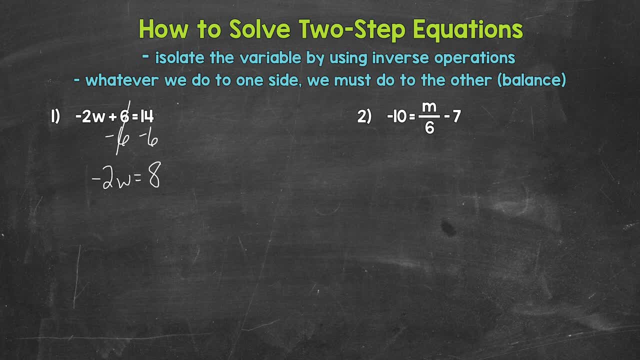 What's the inverse operation of multiplication? Well, division. So let's divide the left side of the equation by negative 2.. Whatever we do to one side, we must do to the other. So divide the right side by negative 2 as well. 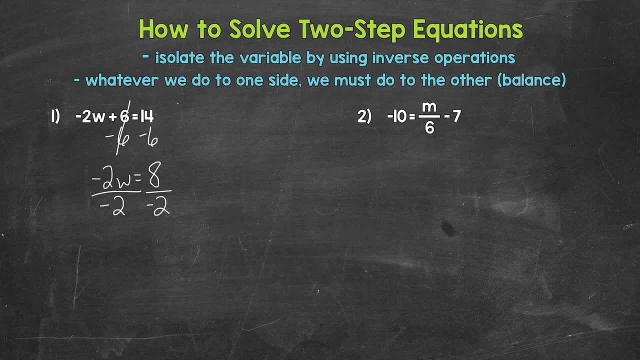 Now on the left side of the equation, we are multiplying by negative 2. And dividing, So we have 8 divided by negative 2. So these negative 2s cancel each other out. W is now isolated, So we have w equals. 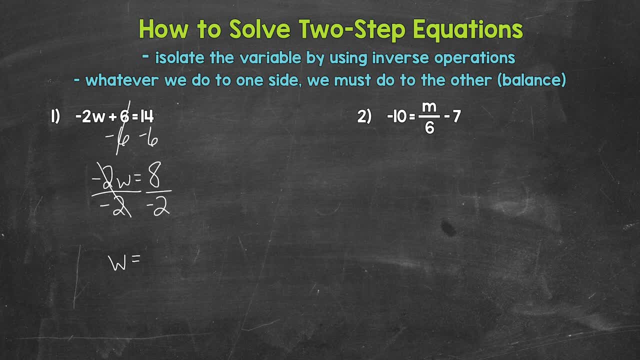 And then on the right side of the equation, we have 8 divided by negative, 2. So we have a positive, Positive, 8 divided by a negative, Negative, 2. When we divide a positive by a negative, we get a negative. 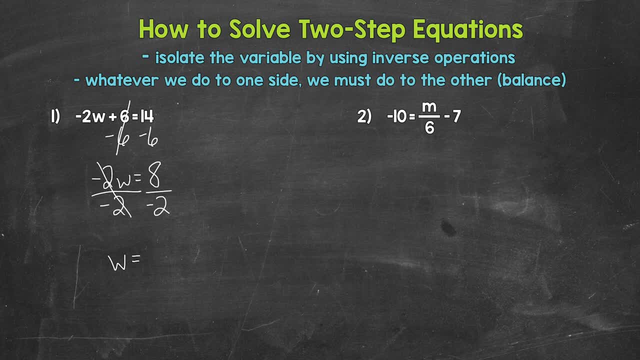 So 8 divided by negative 2. Gives us, Gives us Negative 4.. So we need to be careful there. when we have negatives involved, W equals negative 4. And that's our solution. Now we can check this by plugging negative 4 in 4w. 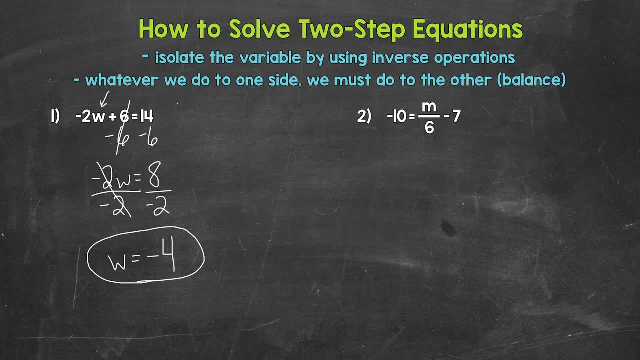 And seeing if it works. So let's do that. So we have negative 2.. Let's come to the side here. Times Negative 4. Plus 6. Equals 14.. Alright, let's start with multiplication. 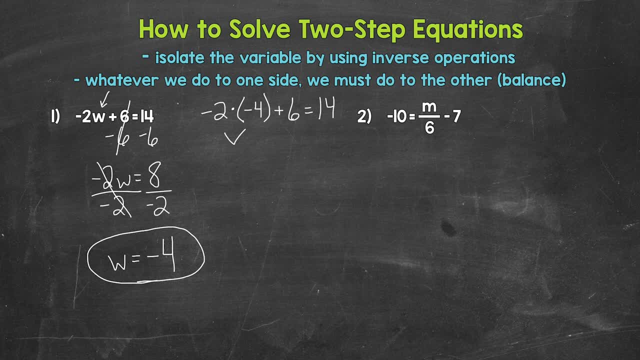 So we have negative 2 times negative, 4. A negative times a negative equals a positive, So this gives us 8.. And then we have 8 plus 6. Which is 14. So we are correct: W equals negative 4.. 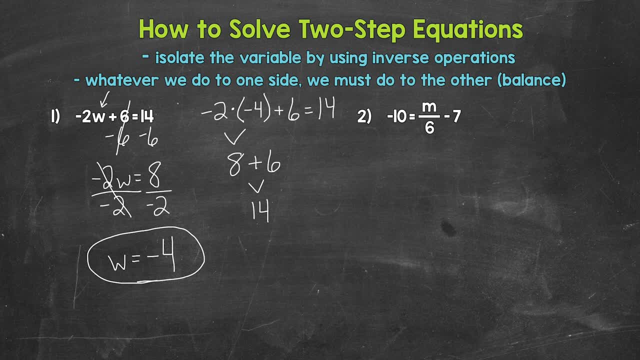 Let's move on to number 2. Where we have Negative 10 on the left side of the equation Equals, And then on the right side we have M divided by 6 minus 7.. So what divided by 6 minus 7, equals negative 10.. 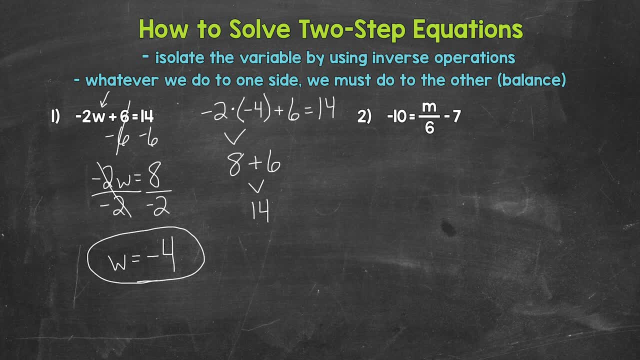 So we need to look to isolate that variable of M. So, taking a look at that side of the equation, We need to undo the subtraction first, So we have minus 7.. What's the inverse operation of subtraction? Well, addition. So let's add 7 to the right side of the equation. 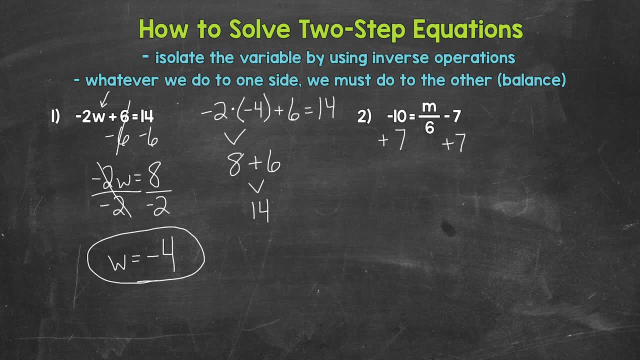 Whatever we do to one side, We must do to the other. Now, on the right side of the equation, We are subtracting 7 and adding 7.. So these 7's cancel each other out. So now we have M Divided by 6.. 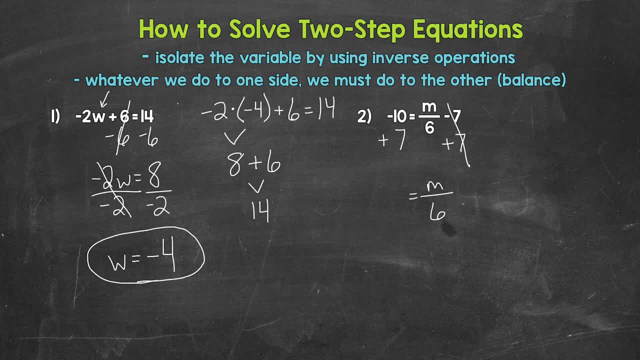 Equals. And then on the left side of the equation We have negative 10 plus 7. So we are starting at negative 10. And we are adding a positive 7. So we are increasing in value by 7. That gives us. 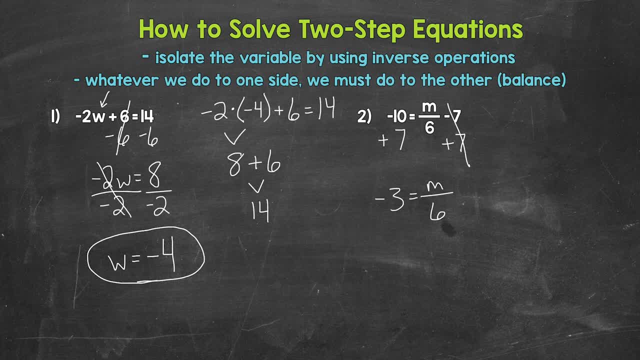 Negative 3.. So now we have M divided by 6. Equals negative 3. So let's isolate that variable of M. We are dividing M by 6.. So what's the inverse operation of division? Well, multiplication. So let's multiply. 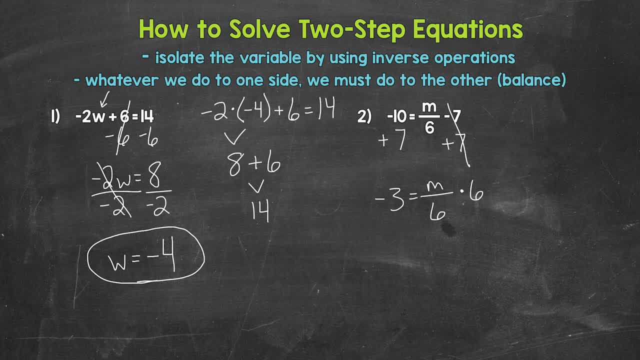 That side of the equation by 6.. Whatever we do to one side of the equation, We must do to the other. So multiply the left side by 6 as well. Now, on the right side of the equation, We are dividing by 6.. 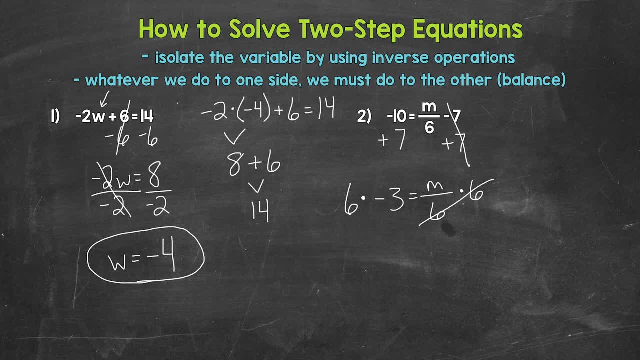 And multiplying by 6.. So these 6's cancel each other out. M is now isolated, So we have M Equals And on the left side of the equation, 6 times negative, 3. Well, we have a positive times a negative. 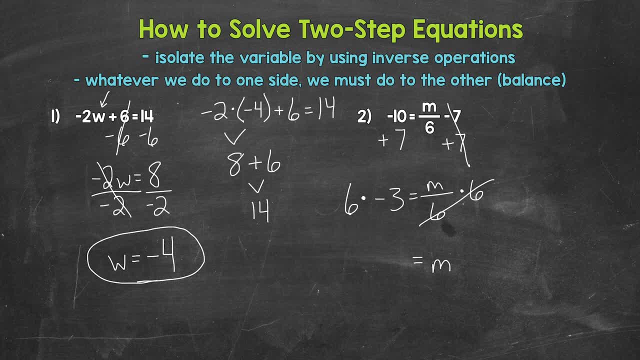 A positive times a negative. Gives us a negative. So 6 times negative. 3. Gives us negative 18. So M Equals negative 18.. And that's our solution. Let's check it by plugging negative 18.. In for M. 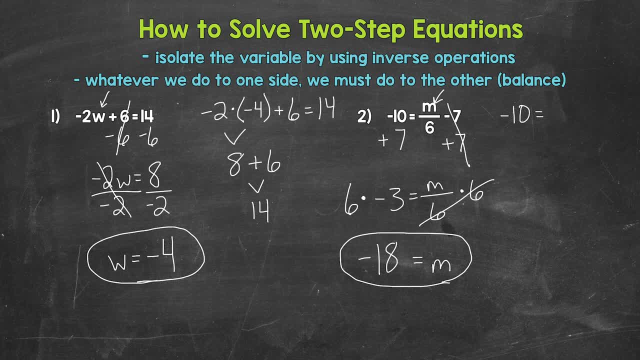 So we have negative: 10. Equals Negative: 18. Divided by 6. Minus 7.. Let's start with division. So we have negative: 18. Divided by 6.. A negative divided by a positive Equals a negative. 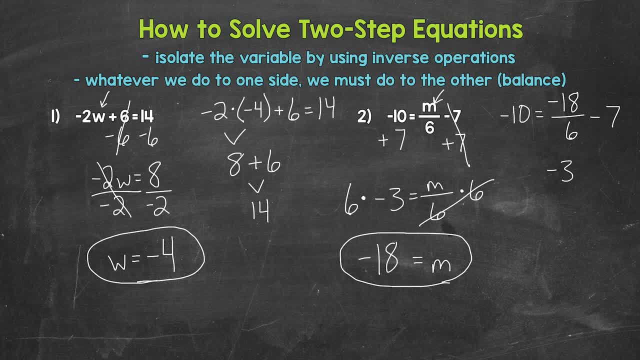 So that gives us negative 3. And now we have negative 3. Minus 7.. Now there are a couple different ways to think through this. So we are starting at negative 3. And subtracting 7.. So we are decreasing in value by 7.. 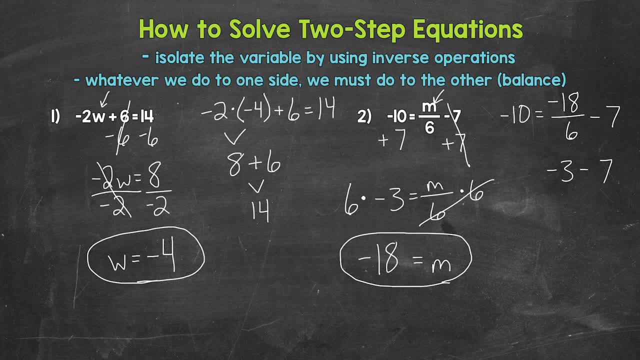 That gives us negative 10.. Another way to think through this: Whenever we have subtraction, We can add the opposite, And that will give us the correct answer as well. So add the opposite, So we have negative 3 plus negative 7..